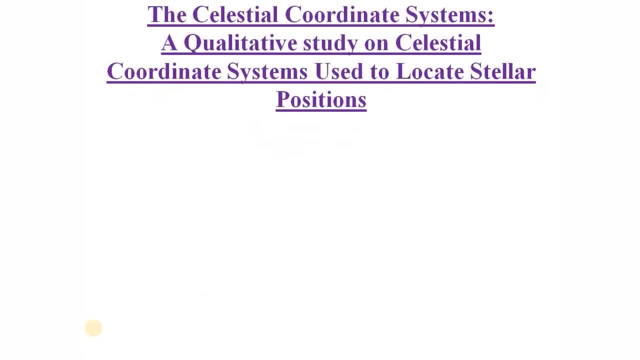 heavenly objects. Okay, So basically we will be talking about celestial coordinate systems, different types of celestial coordinate system and what are the naming done in coordinate systems and what are the origin taken, what are the references taken and, with the references, how coordinates? 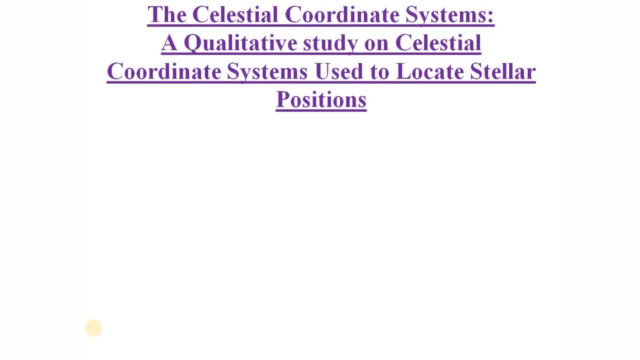 are measured and other matters. So, and the, as you know, coordinates are used to locate objects or points. In ordinary mathematics, we will talk about coordinate system, where coordinate systems are usually used to designate a point or an objects in a 2-D or 3-D space. okay, So usually either in 2-D plane or 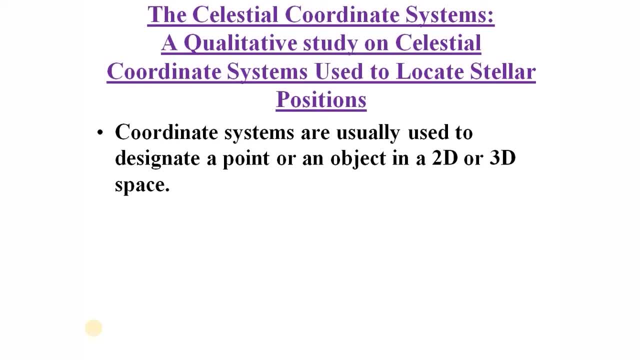 in a 3-D space start using a three dimensional coordinate system which can represent a point, a vertical plane or a arenal plane, etc. else, and how these two objects, X or Y, are represented space also. so when we come to astronomy, but also we deal with average objects. so position of 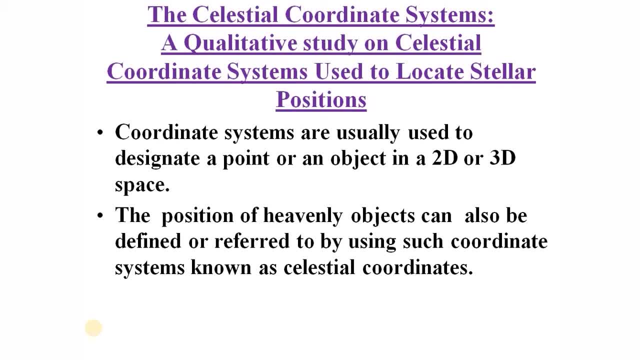 heavily. objects can also be defined or referred by using such corner systems, so that is known as celestial coordinates. okay, so for tracking the motion of objects- maybe a satellite, maybe a planet, it may be an asteroid or comets or anything like that. so in order to track them, 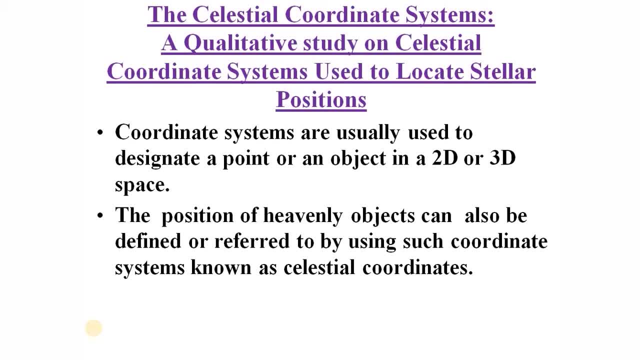 we need some unique coordinate system. only then we can transfer the observation to some other person or, if you want to record them, the coordinates or the presence of an object. we need some reference right. so essentially these are reference frames, okay, used to locate objects in space. so 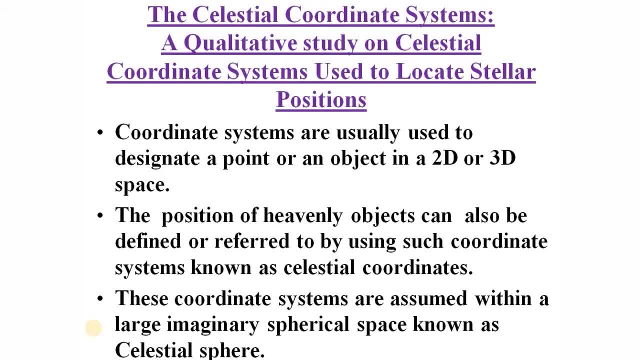 and these coordinate systems are actually assumed or imagined within a large spherical space. okay, so you can. we need some space to imagine a reference system or a coordinate system if you want to imagine them. we need a space. that space here is taken as a spherical space, so that imaginary spherical space is called the celestial. so let us see a few more details of a. 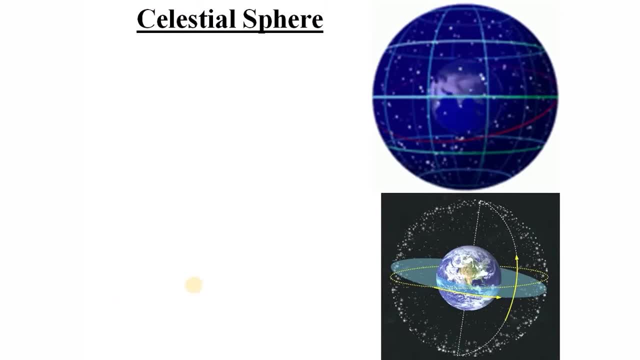 celestial space. okay, so for that consider the figure one. here you can see the earth, it is revolving. and suppose you are standing on earth and observing the sky. what you usually feel? you usually feel that all the objects in the sky, in the space, are pasted on some spherical surface. this is a usual feeling, it's an apparent feeling. 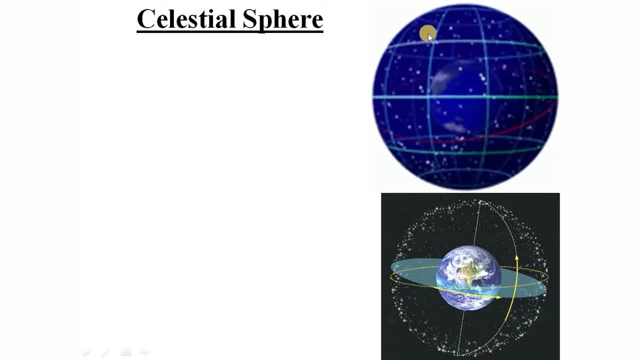 it's everyone, every common man gets when you observe the sky. All objects are pasted or sticking on some surface, So that surface we can call as a celestial surface or a celestial sphere. Okay, so a video object is helped to be located on some on a spherical sphere. 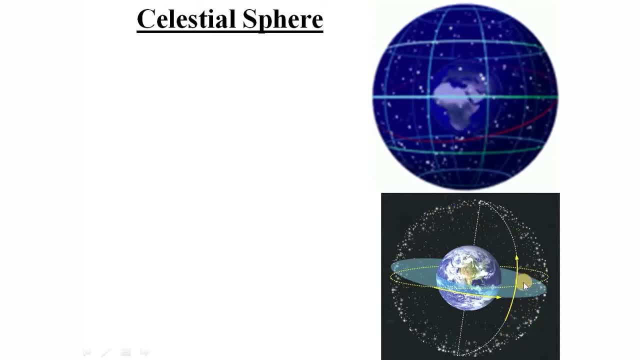 Okay, here also you can see that in the figure 2, some shining objects you can see. So it is a visual, artistic impression of the celestial sphere. At the center we have the earth. Earth is here and all other objects seem to be existing on a surface, spherical surface. 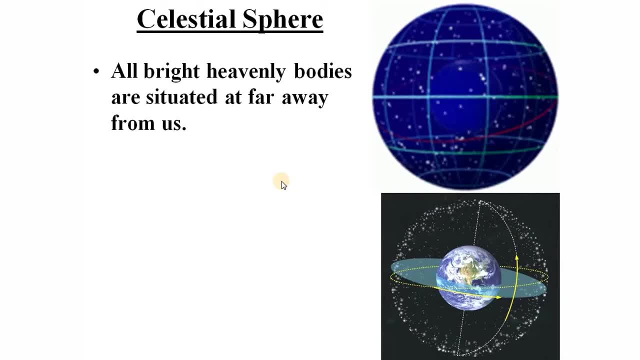 That spherical surface is called a celestial sphere. So all bright and heavenly bodies are situated and far away from us. but all of us are there And all of them, all such objects appear to lie in the celestial sphere, In the surface of a large sphere of infinite radius, whose center is at the observer's eye. 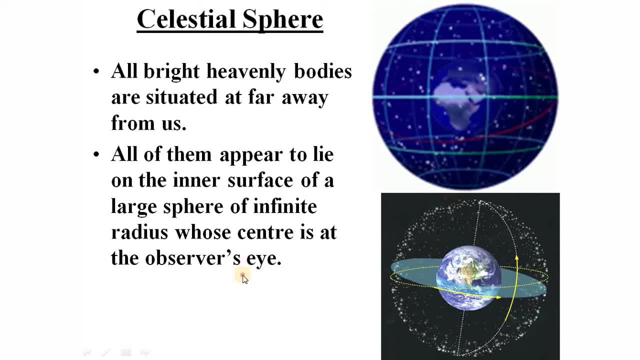 Okay, here center is taken at the observer's eye, Every object is seen to be on the surface. That apparent sphere, or imaginary sphere, is called celestial sphere. I hope you got some idea about the celestial sphere. It is imaginary, still it is very. this concept is very helpful in locating objects in the space. 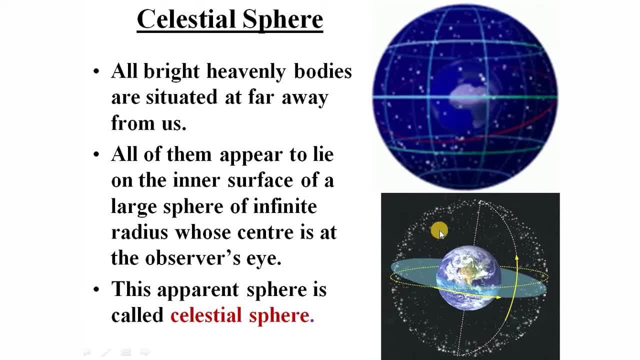 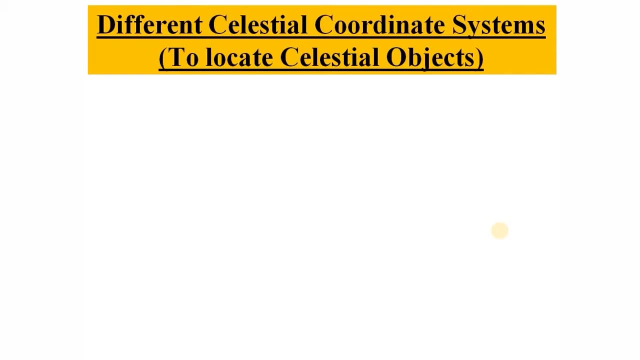 Okay, Without imaginary sphere, it is very difficult to locate them or refer them, or to transfer your knowledge to somebody else. Okay, So that is why we have such a concept of celestial sphere. Okay, So now let us move on to the coordinate system. 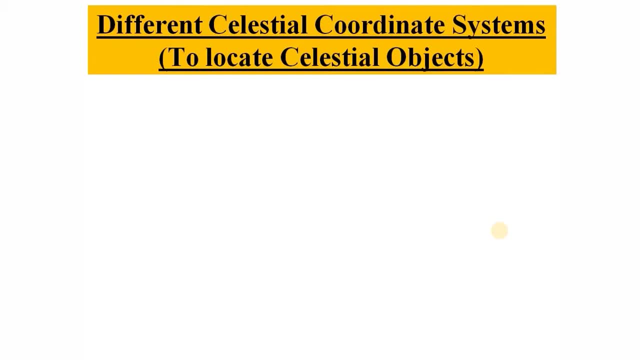 These different coordinate systems are there From time immemorial, or you can say ancient times itself. people felt the need of assuming some coordinate system So that objects in the space can be located or referred very easily. Okay, So during the period of time, many such coordinate systems were evolved. 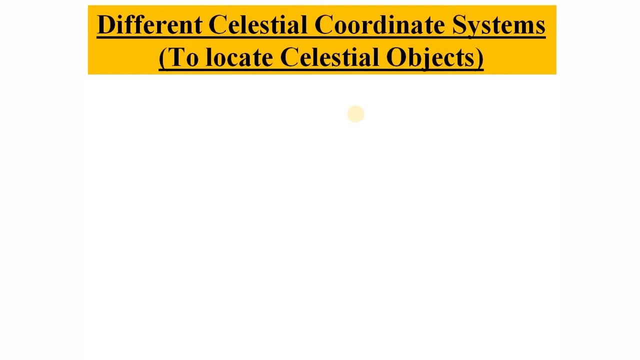 Some of them were both obsolete or useless, So that were discarded And some model systems were developed And now we have very advanced coordinate systems. Let us see few among them. The first one is called horizon coordinate system. We will talk in detail about horizon coordinate system very soon. 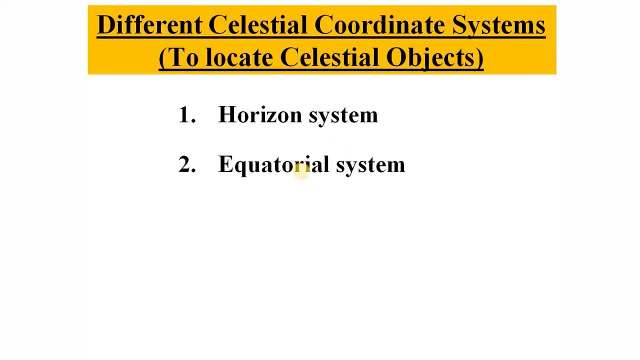 And the second one is called equatorial system. This is also a coordinate system. Every term has its own meaning: Evolution, we will talk in brief. And the third one is called ecliptic system or ecliptic coordinate system. And the fourth one is called galactic system. 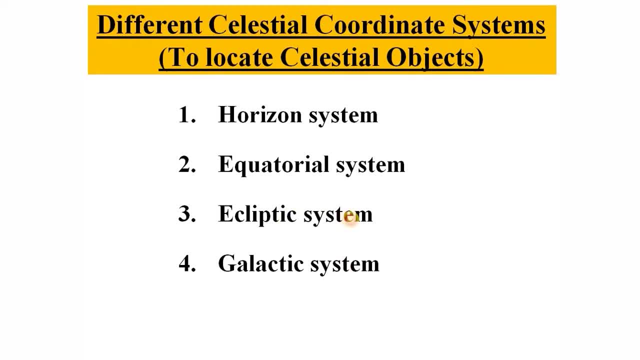 This is much more advanced than the earlier three, And we have the latest one, called supergalactic system. Okay, These are the five major coordinate systems used to locate extraterrestrial objects. Okay, So out of which we will be in today's session, we will be interested to talk about the first three one. 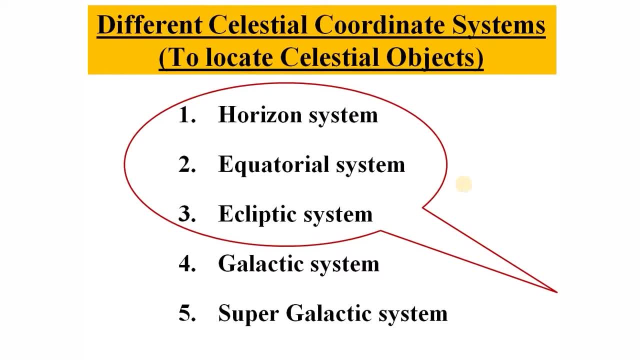 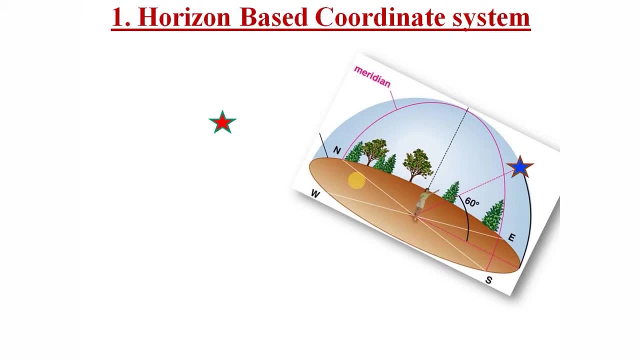 Okay, These are the major coordinate systems used to locate objects from the earth. So we will be focusing on the three First three systems. So right into the stop. Okay, So come with the horizon Horizon based coordinate system. You have the, you have the idea of horizon. 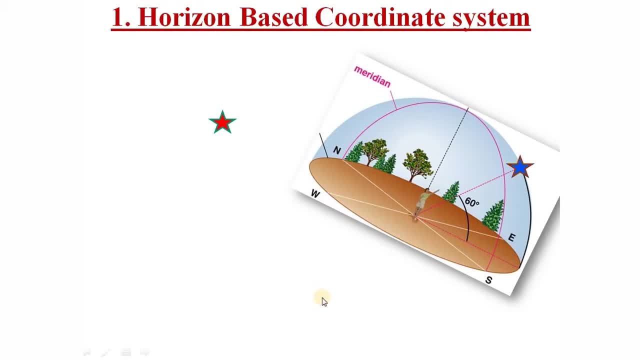 In Malayalam we call it Chakravallam or something like that. Suppose you are standing on the earth. Suppose you are standing on a vast plain ground And you looked at far away objects, What you feel? you usually feel that the surface is extended to infinity, or you can have the 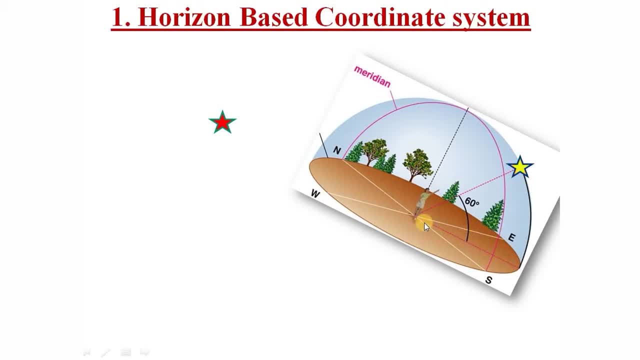 same feeling when you are standing nearby a beach or a seaside and you look at a faraway point. what you feel? you feel that the surface is matching with some celestial sphere. Surface is merging with the celestial sphere at the far end, So that means the entire plane is felt to be joining with the celestial sphere at far. 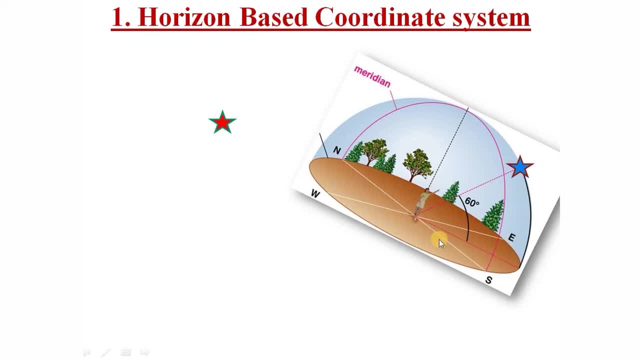 away point. So that plane, the plane, the horizontal plane, intersects with the celestial sphere. also that plane is called horizontal plane and you can imagine a circle. that circle is called horizontal circle. So our first coordinate system is based on this horizontal plane. In the horizontal plane we have a circle. 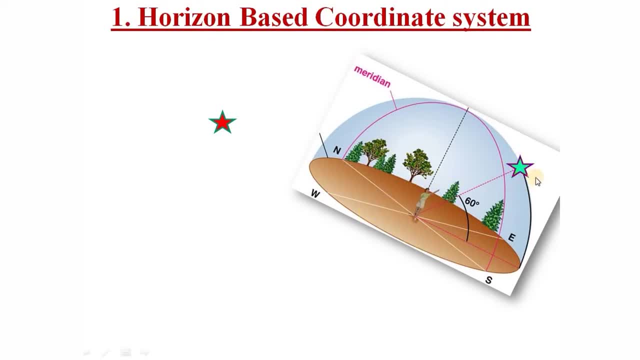 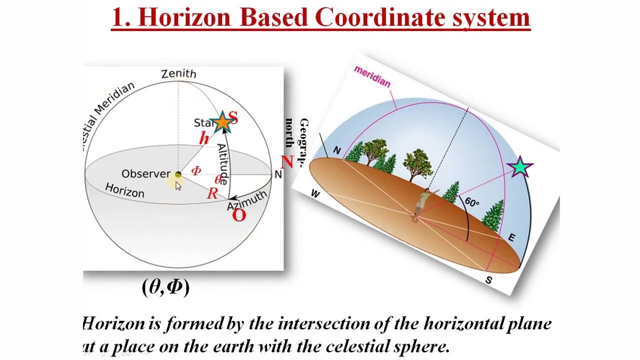 So our first coordinate system is based on this horizontal plane. If you are standing, you can locate any star, and star can be designated with some coordinate. So let us see how this is done. For that you have a sphere here, celestial sphere. this is the celestial sphere and your 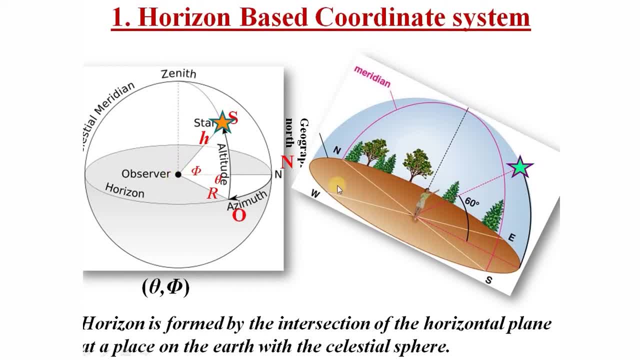 small, tiny earth is here. you can see, tiny earth is here and you are here at that point and you are looking at the star. So then, how origin is taken From this coordinate system is given at the geographical node. geographical node in the. 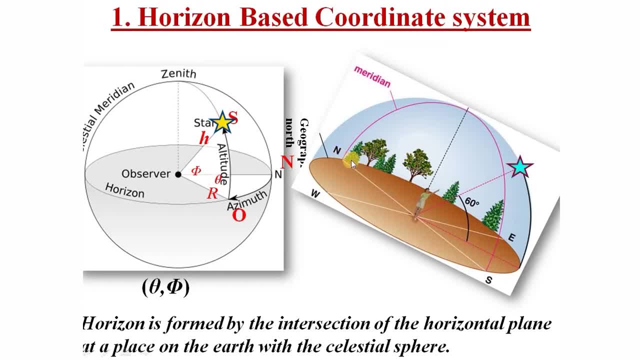 sphere. you can see this is node and you make an angular measurement. So here is your star. you can do a meridian line to the celestial sphere, a meridian line, a line, actually a meridian line like this on the surface, celestial surface. 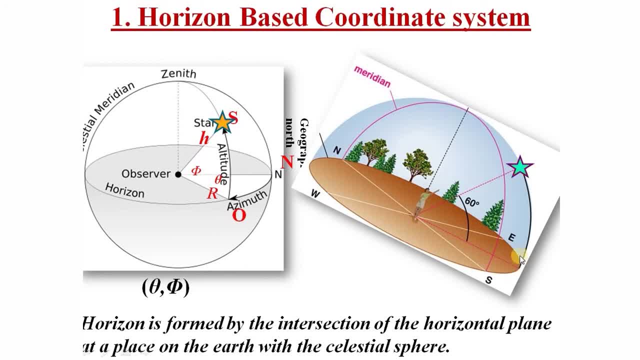 So that line will intersect the horizon plane at some point. So here suppose you mark this point at some point. So this meridian intersect the horizon plane at some point. The angle measured from the geographical node to this point, geographical node to this point. 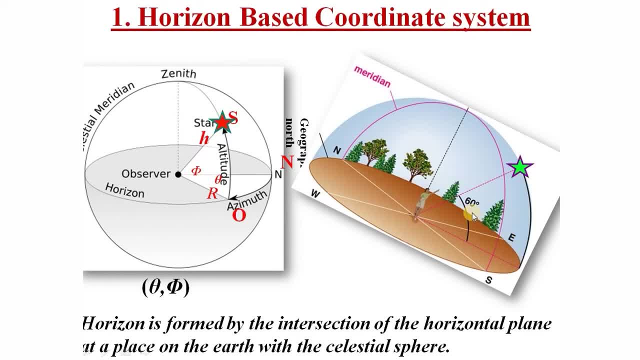 that is the first angle. okay, first angle. You can call it some inclination or horizon angle or something called azimuth angle. actually, That astronomers favorite name is azimuth angle. okay, Azimuth angle is one of the coordinate, Again, to reach. in order to reach the star, you have to move, like this in the meridian. 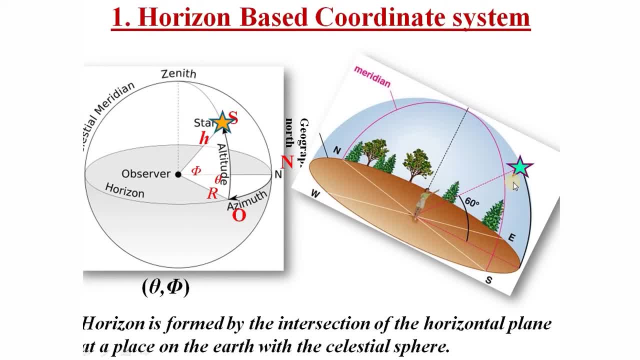 plane also. So that angle is called the altitude angle, altitude. okay, So altitude is the second coordinate. So this way, using azimuth angle or azimuth and altitude angle or altitude, you can locate the star in the sky. okay, So this is the method by which star is located. 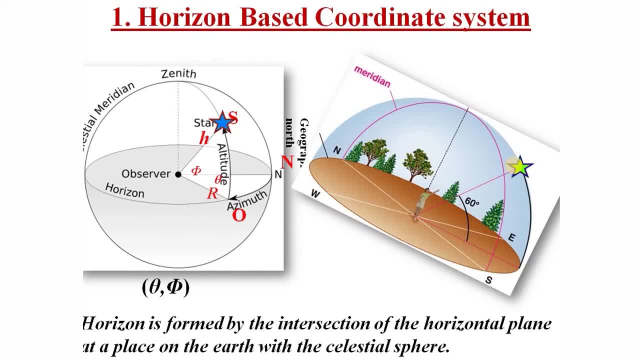 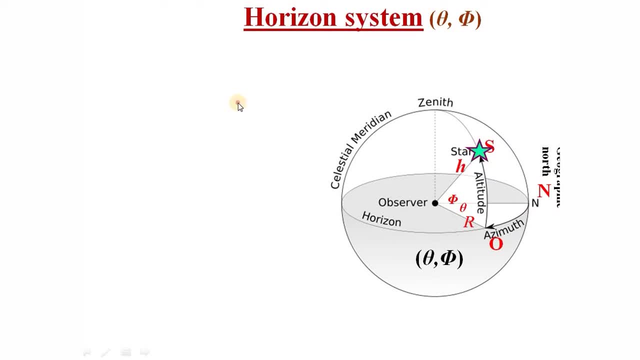 Okay, So in the horizon based RDA system- Understand. I hope the idea is clear. Let us sum up once again what are done in horizon system. Here, geographic north is the origin of the horizon. Your measurement begins from geographic north, Measurement starts. So, first thing, and secondly, 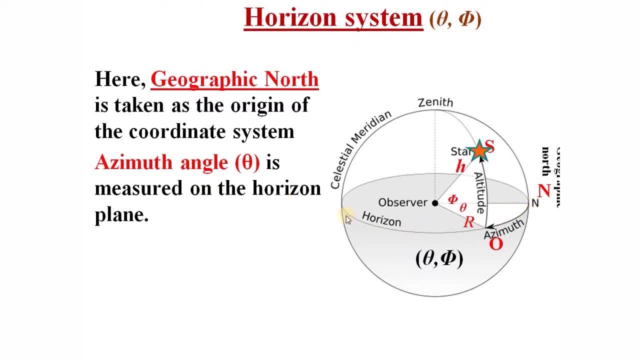 azimuth angle is measured on the horizon plane. So this is the horizon plane, as you know, and your angular measurement is done in this plane. So that angle is azimuth angle. This is designated as a theta and the second angle is called altitude angle and that is measured. 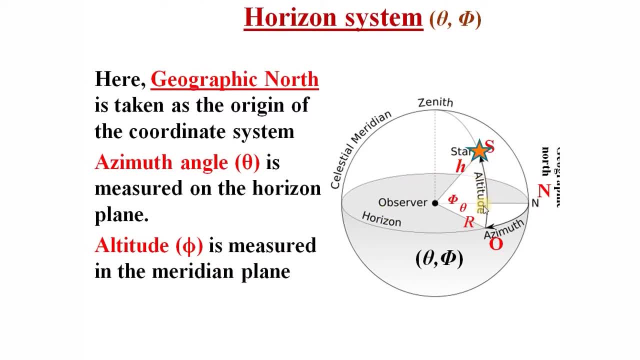 in the meridian plane. Okay, In the figure you can see this is the meridian plane or altitude angle. So two angles measured. Angles are usually measured in degrees. You can also measure. degree can be again subdivided into minutes. Minutes can be again subdivided into. 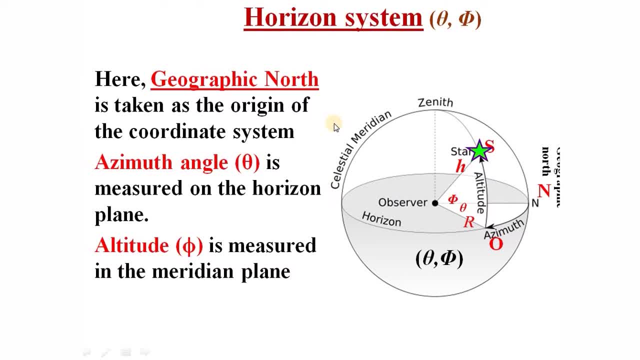 seconds. So for minute measurements you can use seconds also. Okay, So that is usually required. So angular measurement done in degrees, minutes and seconds: Okay, So that will help us to make measurements more accurate. accurate in size. So now let us come to the 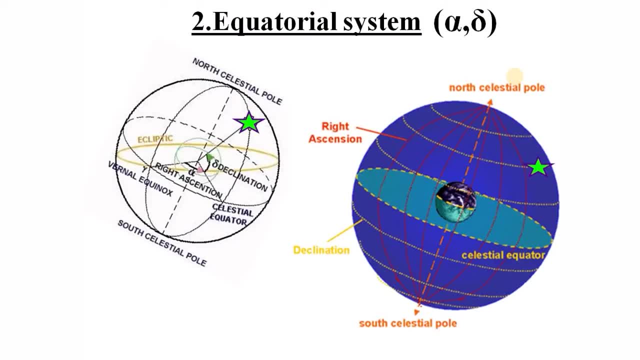 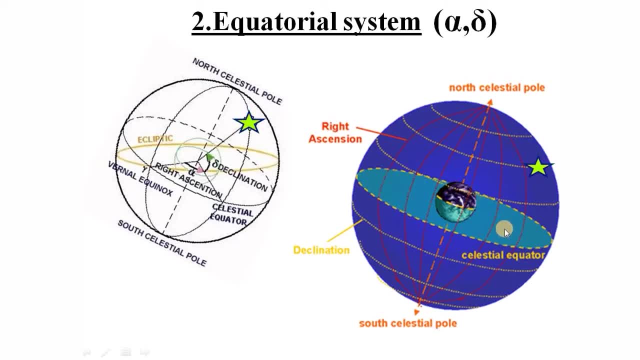 what is equatorial? actually, Equitorial plane that is coming out of the world. equator, You know, the longest tail latitude on the earth is called equator. Okay, This is our earth, as you see, and this is equator at the middle, If you imagine a extended surface, extended. 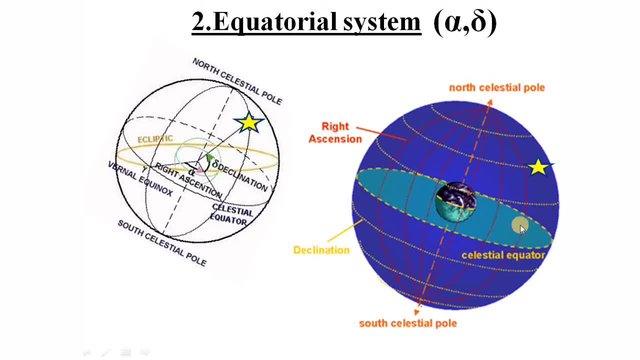 this surface parallel to the equator. this is the extended surface. the blue surface that you can see is the extended surface parallel to equator and in the figure you can see that this extended surface intersects with the celestial sphere. this is our celestial sphere and this extended surface. 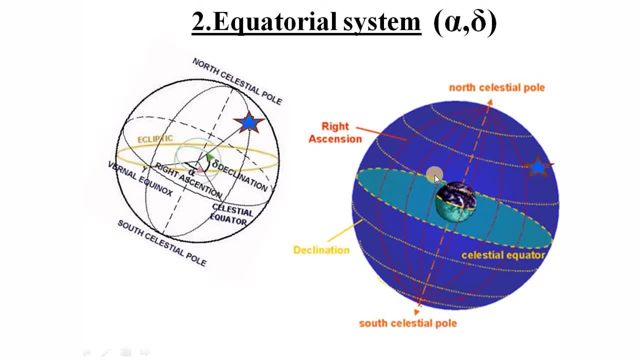 intersects with celestial sphere, so that intersecting plane gives you something. okay, this circle is called the celestial equator, this circle is called celestial equator and this plane is the equatorial plane. so we need this plane here to make the measurement, our coordinate system. in the previous topic we took the horizontal plane as a reference plane. we had a plane there that 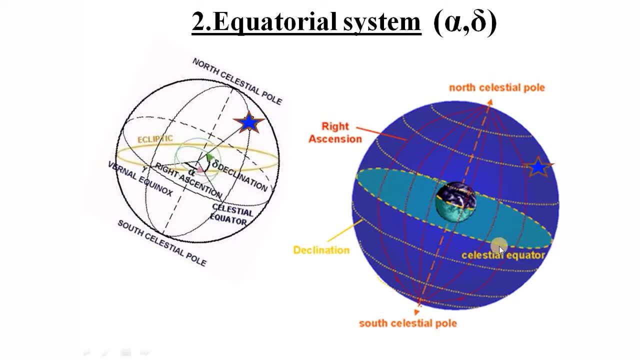 was the horizontal plane. similarly, here the plane is the equatorial plane, or we can say celestial equatorial plane. okay, this is that and that is required for our measurement. first plane, and in order to make an origin, you need an origin. also, our measurement should start from the origin. 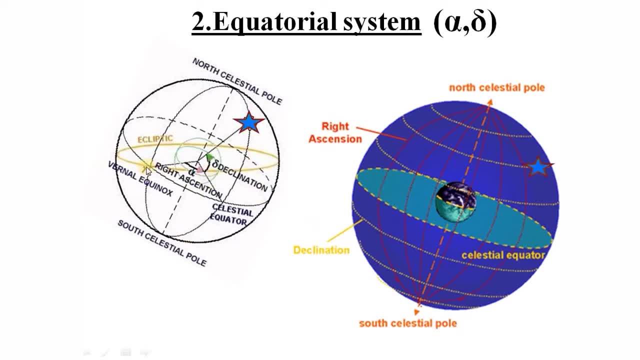 how that origin is taken. origin is taken as the vernal equinox. so you know what is a vernal equinox point. how do you get a vernal equinox point? you can imagine two planes. one is the equatorial plane and the equatorial plane, and the equatorial plane is the equatorial plane. 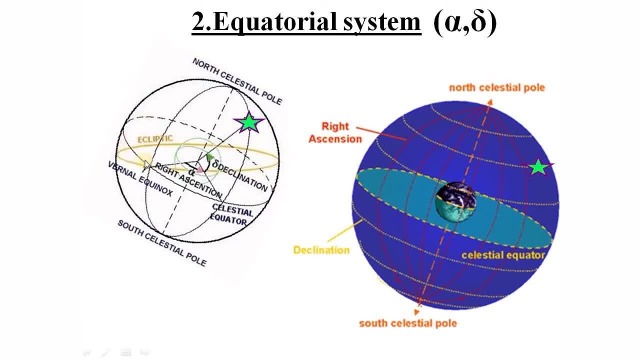 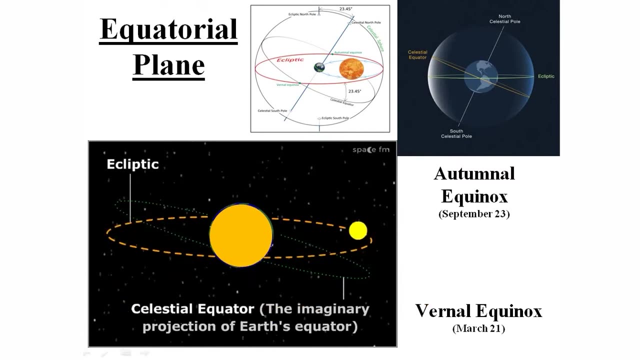 one is the eclectic plane. okay, two, two planes are the one is the equatorial plane, one is the ecliptic plane. then question arises: what is an ecliptic plane? okay, ecliptic plane. we can easily find out how. how do we find the ecliptic plane? ecliptic plane is that plane in which earth moves. 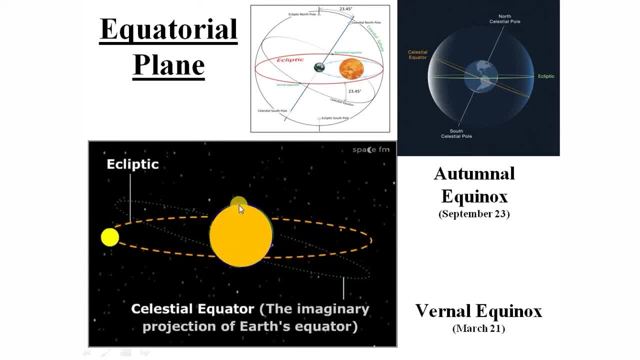 around the sun. from the figure you can see this graphics. you can see that equatorial plane and equatorial plane are not. same plane is shown in the green dots, whereas the clitoral plane and the ecliptic plane is shown with this dashed lines. okay, they are not parallel and instead they intersect. okay, so you get. 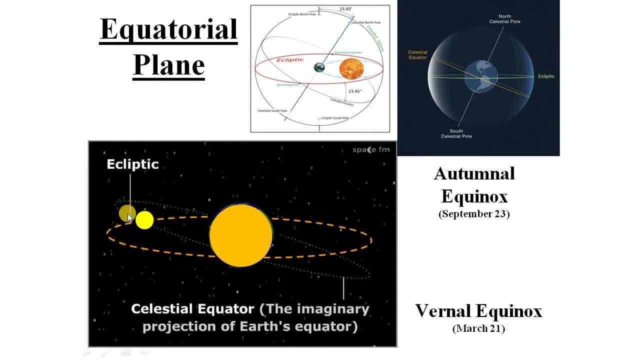 the two intersecting point. the ecliptic circle and the clitoral circle intersect at two points. so you get two, two points. the first intersecting point we call as vernal equinox and the second intersecting point we call as abdominal equinox. the first intersecting point is our side, the 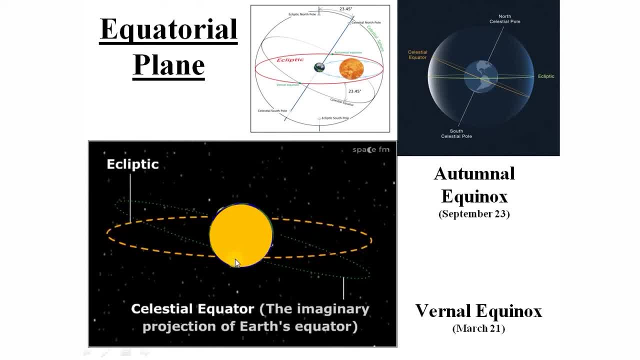 front side. and you know, at vernal equinox what happens: sun will be exactly top of the equator and we have equal day and nights, and it usually happens at 2.00 am to 3.00 am and 3.00 am. it is normal, and so we get two linear intersecting points that we call as 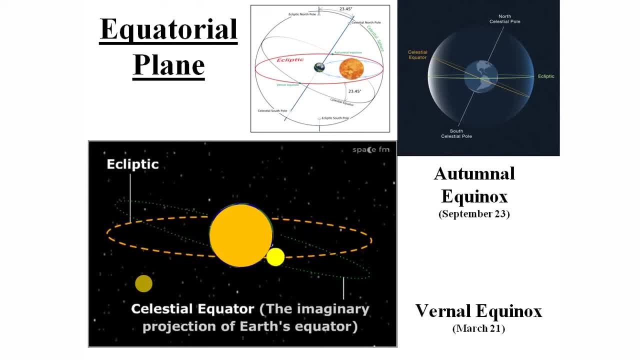 24th March, and on the other side we have the terminal equinox, again the Sun comes on the top of equator and again we get the equal day and night. so these are all well known to us. we are more concerned here with the vernal equinox point. okay, vernal equinox point is: 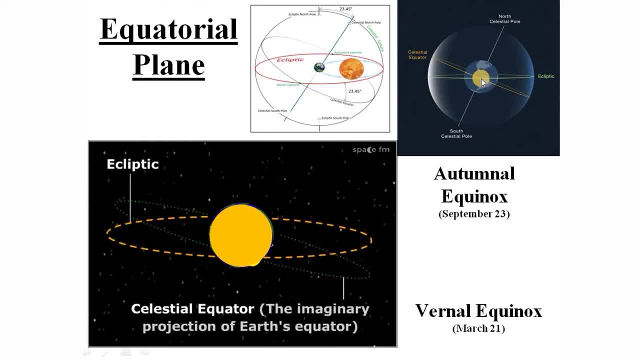 here that is taken as the origin of the equatorial system. okay, origin where we start our measurements. so measurement is taken from vermal equinox point along the equatorial plane. So let us see how this is done. we have the vernal equinox point shown. 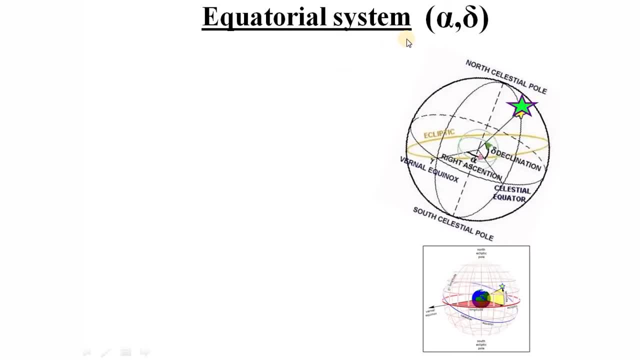 in the figure and també in the Justine and in equatorial system we have the vernal equioral point as the origin and the measurement is taken along the equatorial plane. so this is equitorial plane. So to understand. So to a v envelop we should be looking at in this strip as we are, I can work on Zen. 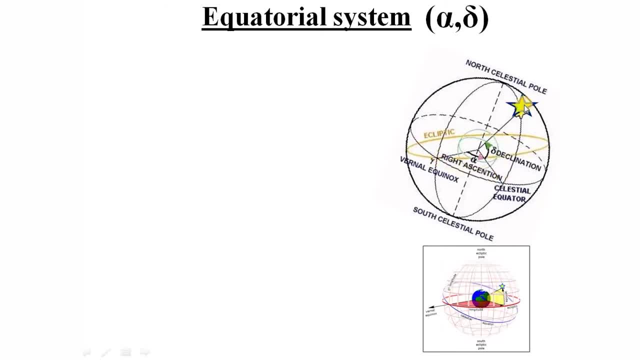 general. you study it. we are the four one where, yeah, 1, 15 v, and then we have v about 0.2. things are there. one is the measurement along the plane. suppose star is here, then you can draw a meridian again. the meridian will intersect the equatorial plane at some point. the angles subsided. 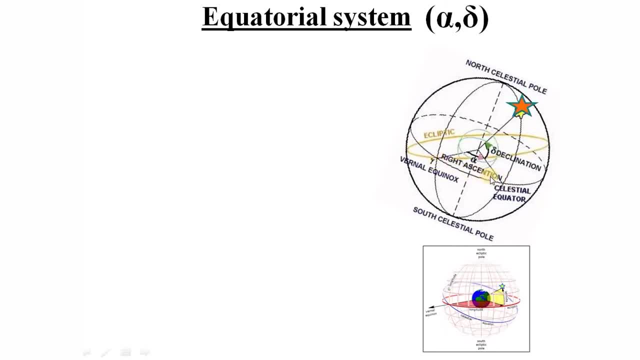 by the intersection from the origin. that is called the ascension. ascension: the angle denoted as alpha, and you have the second angle, measured along the meridian plane, from the intersecting point to the star. that is called the declination. you do not have to be delta, so ascension and 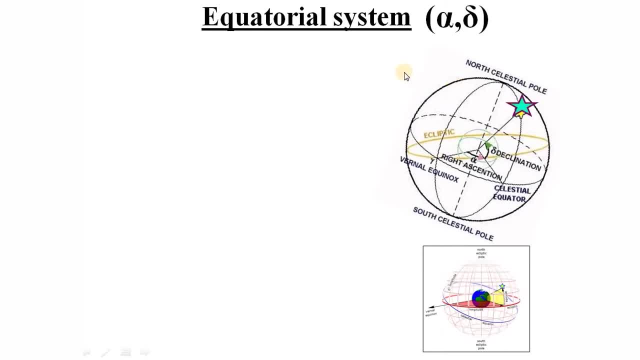 declination are the two coordinates, alpha and delta, to mark the position of a celestial arc points. okay, so let us sum up here. first thing is that vernal equinox is the origin of this coordinate system, as shown in the figure. vernal equinox is here. and second thing, ascension and 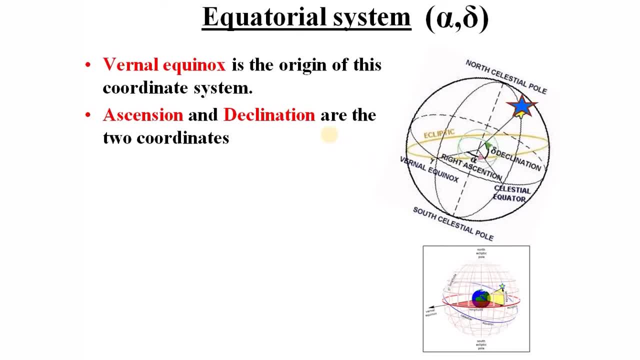 declination are the two coordinates. ascension is also called a right ascension because we are moving the right hold in order to make the measurement so right. ascension is usually used by astronomers and the declination is the angle measured along the meridian plane. so that is shown here. the angular distance from the vernal equinox to the point where 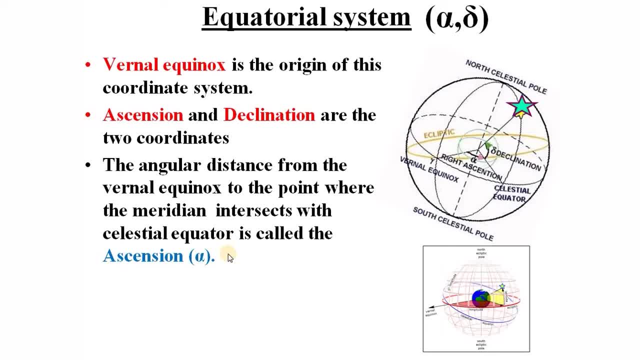 the meridian intersects with the star, so it is called ascension, alpha, okay so. and angular distance between the star and the celestial equator is called declination. so these are the things to be discussed in the pictorial system, the second coordinate system, and usually both are marked. 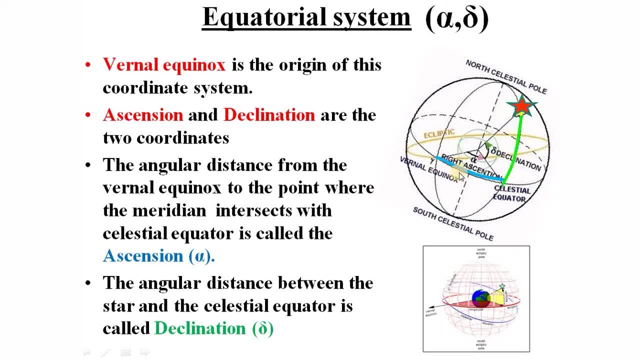 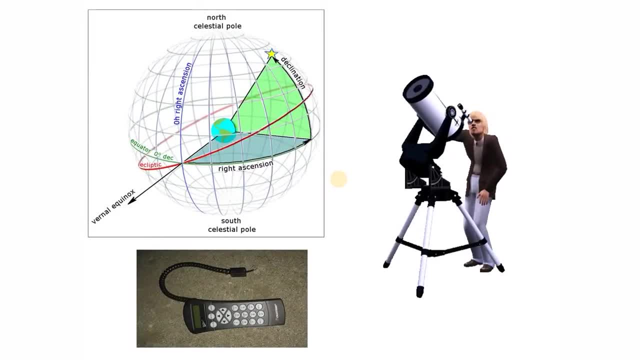 in the figure. okay, it is the declination and it is the ascension. i hope the idea is clear and usually we know in measurements or in telescopic measurement, and either you can use a pictorial system or ecliptic system. also, in many old models even horizontal systems are also used. 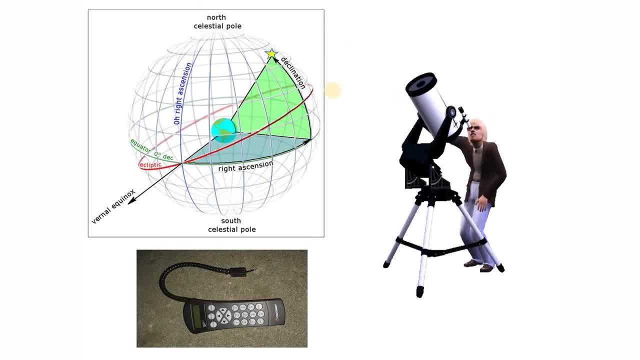 one can select appropriate system for their particular use. in many modern telescopes many coordinate system will be embedded in the in the server. appropriate selection can be done using hand controlled remote. so that is what is shown here. by suitable selection, appropriate measurement can be done and the suitable catalogues are available, published by different astronomical Arab world server. 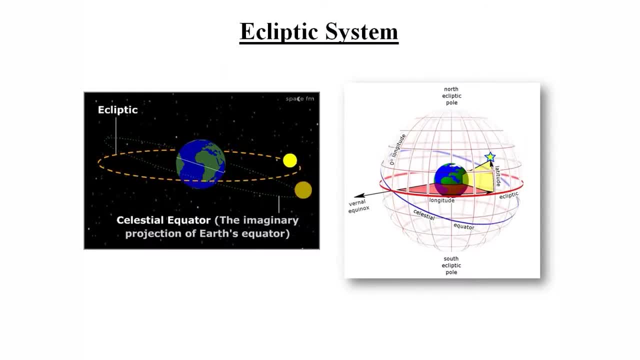 okay, and now let's move to the third coordinate system. that is called ecliptic system, as i already mentioned in ecliptic system And the reference plane that we have adopted is the Euclidic plane. As already mentioned, Euclidic plane is the plane in which the earth moves around the 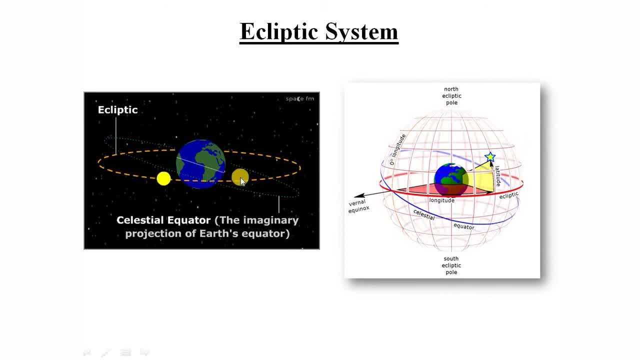 sun. Earth is actually moving around the sun. so there is a plane and measurement is done along that plane. In the figure you can see the red line. that is the Euclidic plane, And here also the origin is taken as a vernal equinox point. okay, 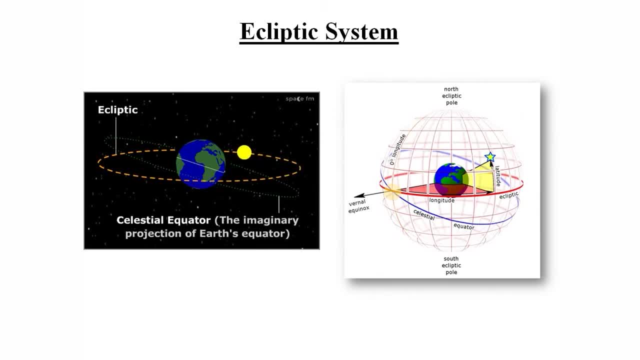 Your measurements start from vernal equinox, just like taking north. whenever you make measurement on the earth surface, we take north, or geographical north of the reference point. In a similar way, in astronomical measurement, we start our measurement from vernal equinox. 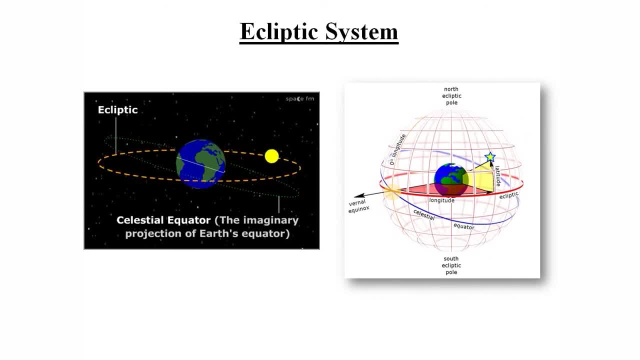 point That is well marked and well understood, the direction is well understood and your measurements start from that. Or any telescope, any standard modern telescope, are well marked and well understood And your measurements start from that. So this is the embedded with idea of vernal equinox direction. 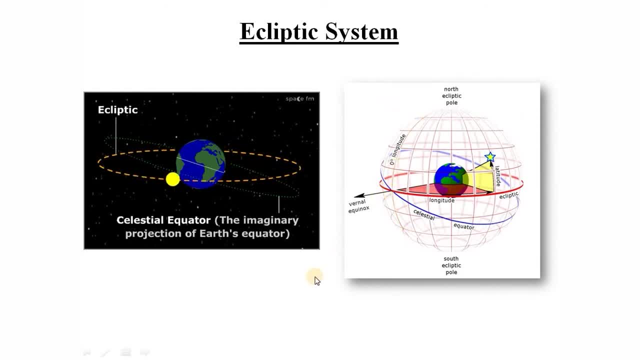 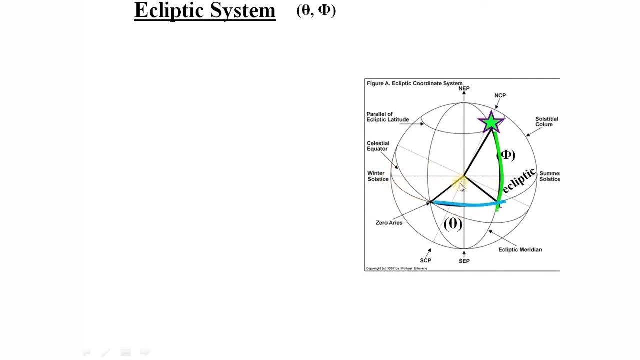 Its orientations are well known to or well recorded in any modern telescopes. Okay, so here, this is the origin of the Euclidic system And in order to make the measurement, we have the Euclidic plane here. okay, Earth is here. do not confuse that. this is the earth. no, absolutely at the center. 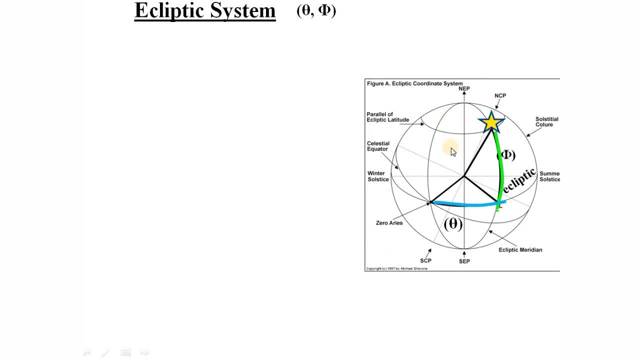 a spot is there, that is the earth. Okay, And this is the celestial sphere. okay, And this is the vernal equinox point, and here measurement is done along the Euclidic plane. okay, So this is the first one. this is called the celestial latitude. okay, celestial latitude. 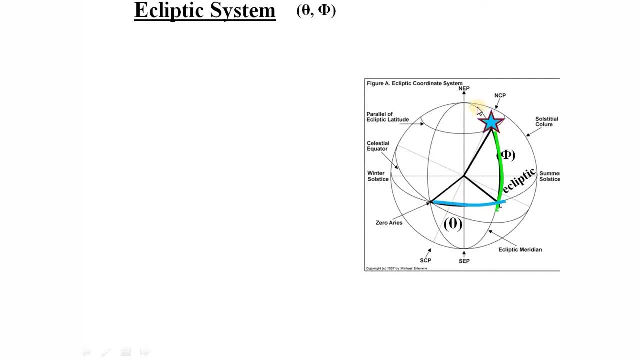 denoted with a theta. okay. And again, a meridian drawn to the star will intersect the Euclidic plane at some point, Euclidic plane at some point. So this substance and angle, Okay, Okay. So that angle is shown here as phi. okay, that is called the celestial longitude, okay. 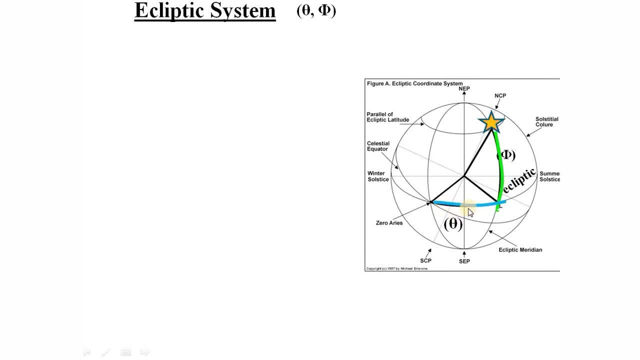 sorry, the celestial latitude. The first one is the celestial latitude and the second one is the celestial longitude. So that is denoted with phi. okay, So idea is clear. let us sum up the idea here. Here also, the vernal equinox is the origin of the coordinate system shown here. 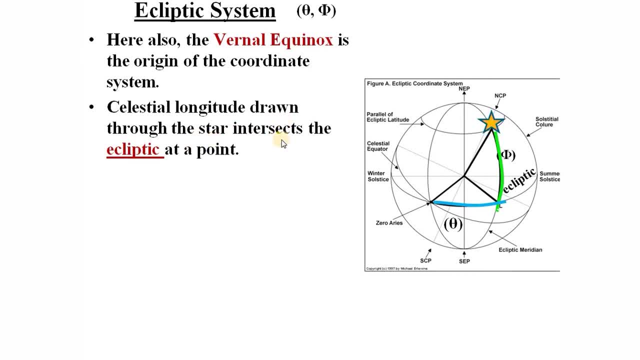 Okay, So the celestial longitude drawn to the star intersects the Euclidic point at some point. okay, So that is shown here. And the angular distance measured from the origin origin is the equinox point. origin to then the second point shown here along the Euclidic plane is called celestial longitude. 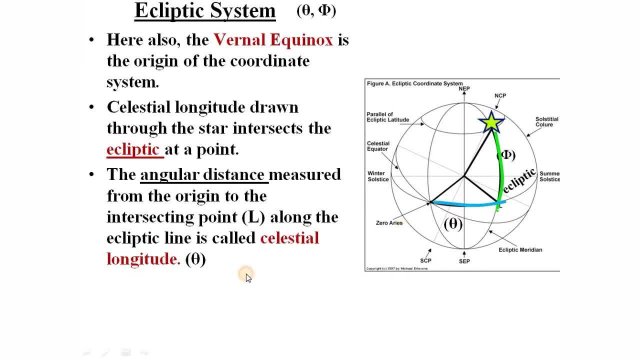 So this is the celestial longitude denoted with theta And you have the second point. Okay, And you have the second coordinate. what is that Celestial latitude? The angular distance measured from the intersecting point to the star to the star is called the. 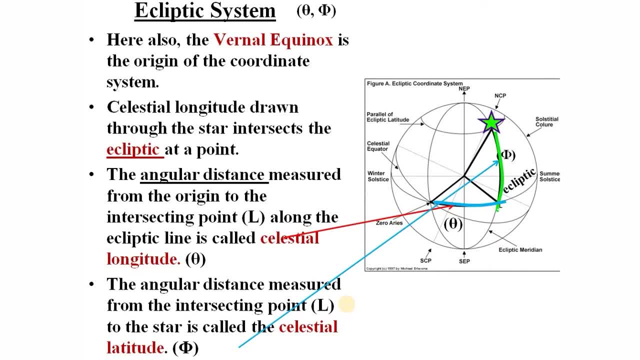 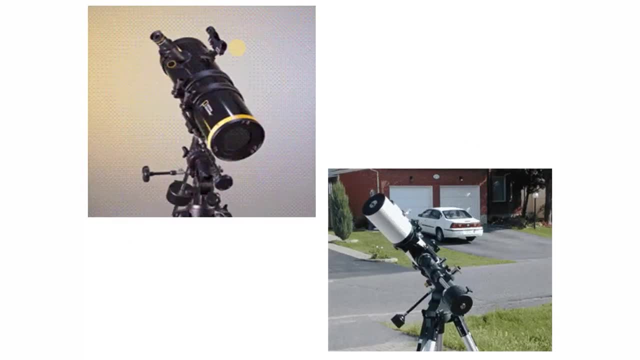 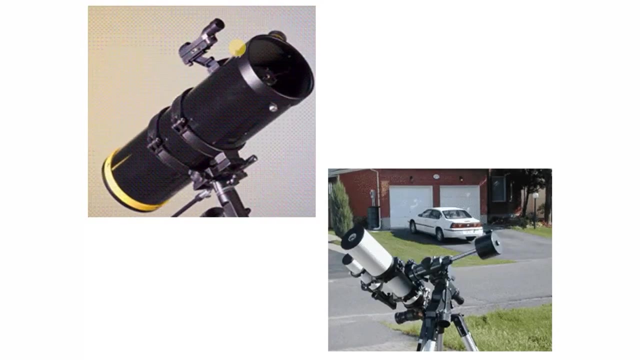 celestial latitude, celestial latitude. So this way celestial longitude and celestial latitude are the coordinates of this thing. ecliptic coordinate system and origin is taken from the vernal equinox. Okay, So I hope the ideas are clear And in modern telescopes, as I already mentioned, appropriate coordinate systems are well programmed. 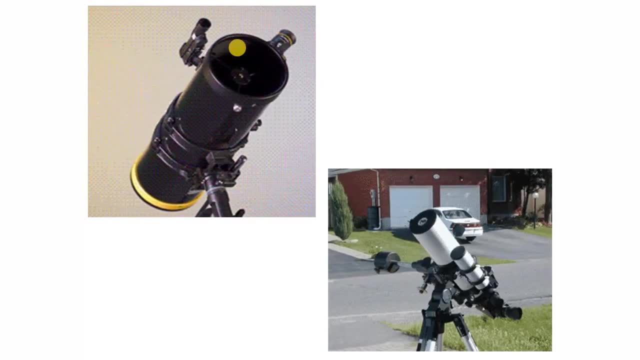 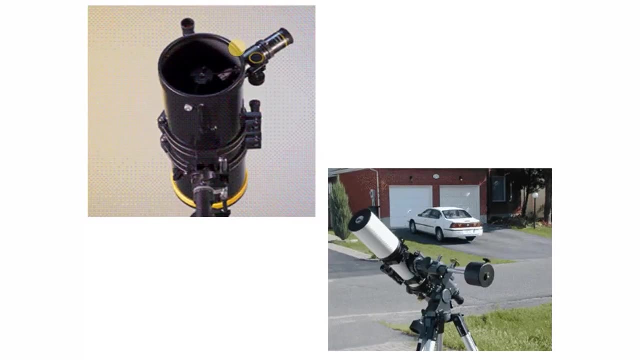 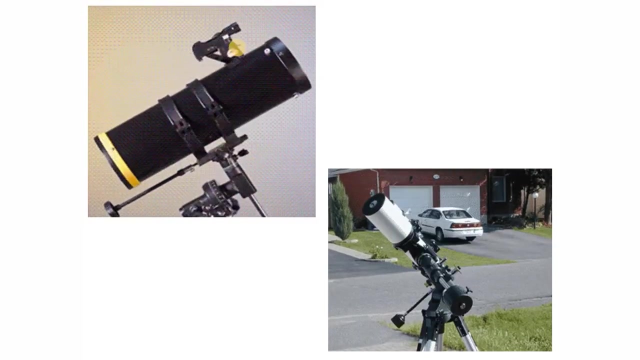 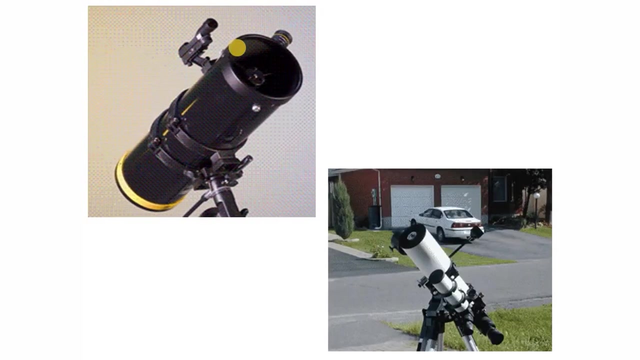 One can select a suitable coordinate system Once you tune a particular heavily object with a telescope. modern telescope have the feature that it can immediately track the motion of the heavily objects. Okay, So when a heavily object is tracked and spotted, telescope will continuously monitor. 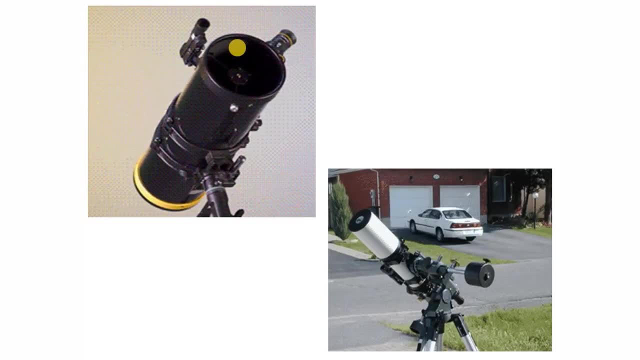 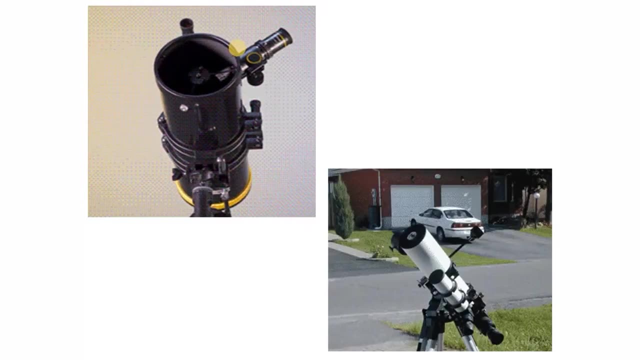 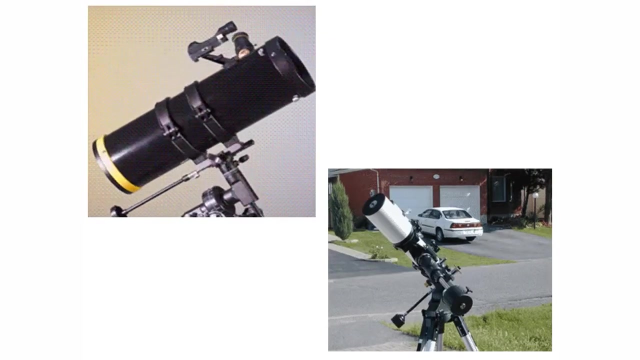 the movement of the object in the space. Okay, This way continuous motion or movement of the object can be properly studied. So such telescopes are available in the market today. One can use appropriate telescopes and do our astronomical observations very wonderfully. 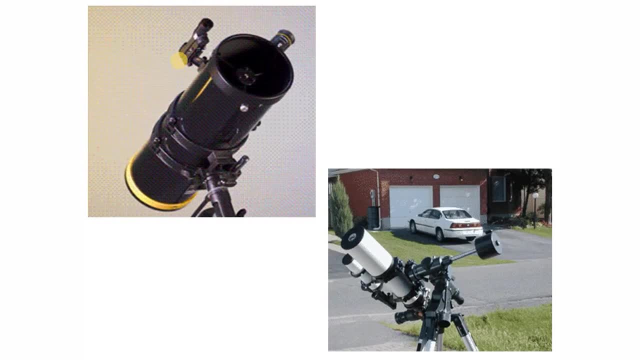 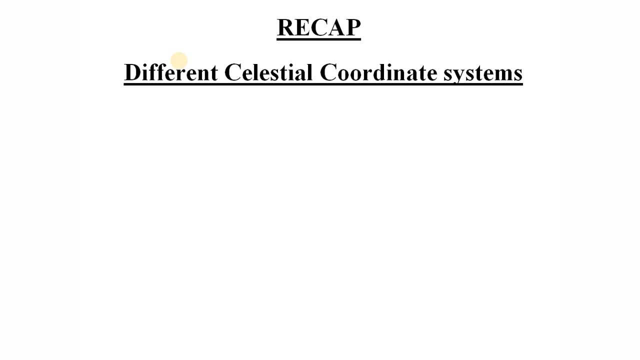 Okay, So these are some of the important points. So once again, let us recap the ideas We studied about different celestial coordinate systems. The first one was horizon system, the oldest one and in which Zuckerman's knot is taken. 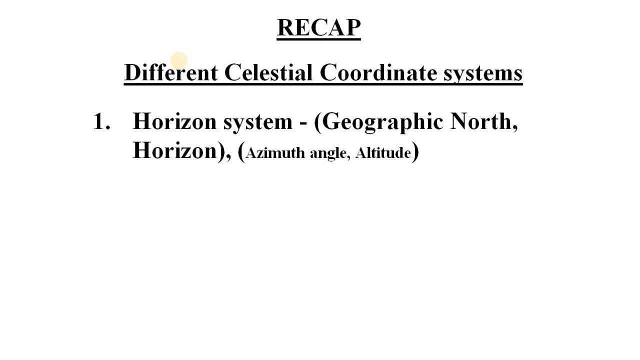 as the origin and azimuth, angle and altitude are the coordinates used to locate objects in the space, And the second coordinate system is the horizontal coordinate system. So these are some of the important points. And the second coordinate system was equatorial coordinate system in which vernal equinox is.